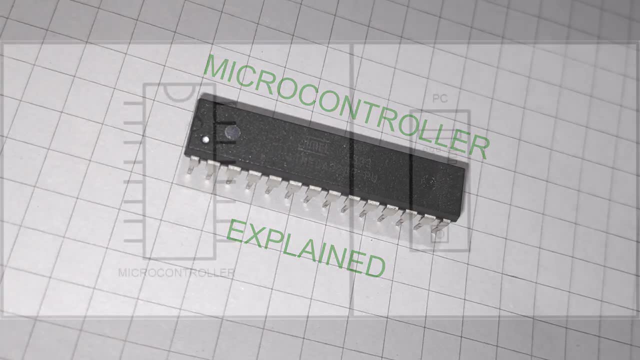 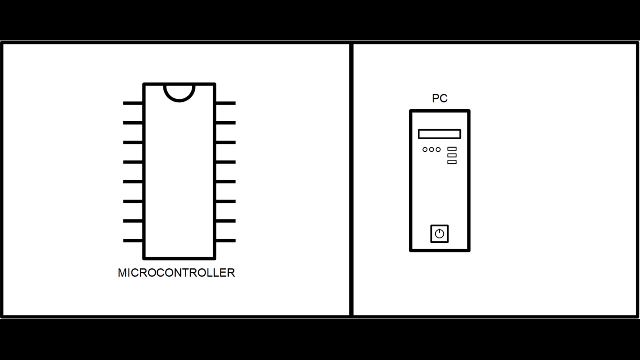 So what is microcontroller and how does it work? Basically, you can think about microcontroller same as you would think about very underpowered personal computer, because they both have a very similar structure. Only, in case of personal computer you have the ports, like CPU memories and serial interfaces separate, where in case 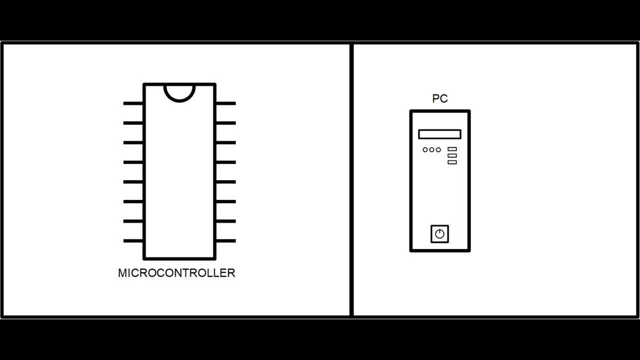 of microcontroller. they are integrated in one chip. Same as you can connect a keyboard and a monitor to a personal computer to input and output some information, you can do it also with microcontroller, only in that case using, for example, buttons and LED lights. 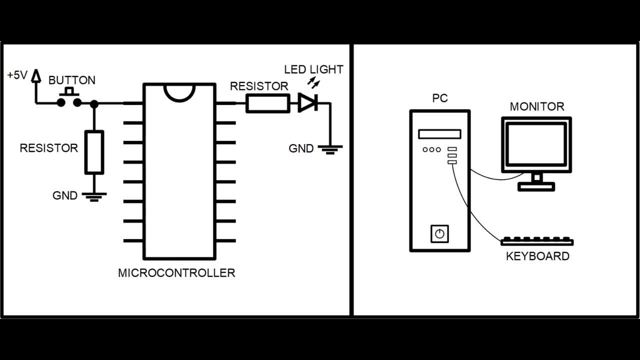 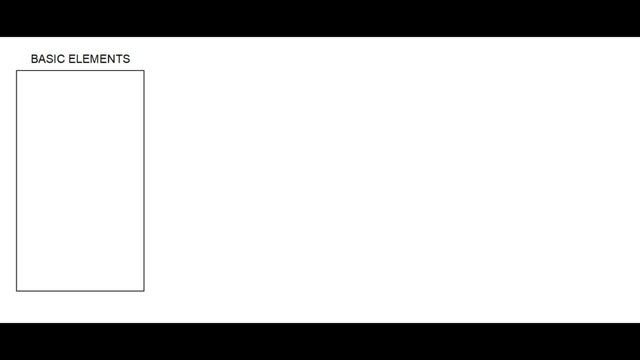 But what exactly is a microcontroller and how it is made? To fully understand that, you have to have some basic knowledge about elements that are used in electronics like resistors, transistors and diodes. Here will be a brief recap. Resistor is used to limit the current that is flowing through the circuit or to create a 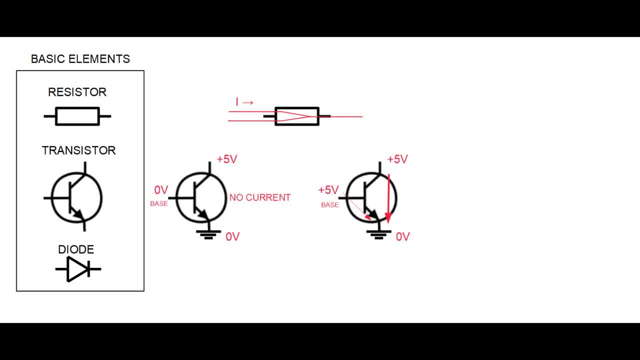 voltage drop. About transistor, you can think same as you would think about some type of valve. In case of a valve to control the flow, you are turning the handle, but in case of a transistor to control the current through the transistor, you are changing the base. 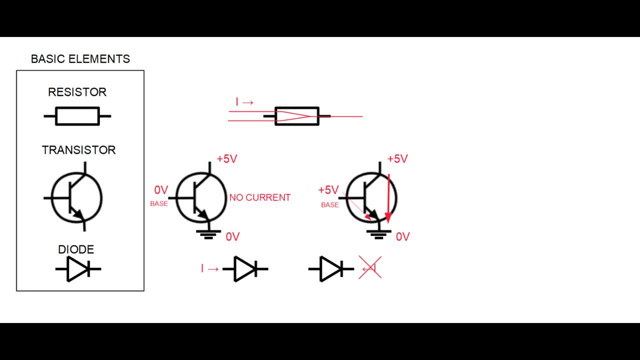 current, And the diode is simply an element that allows to flow the current in one direction, but it blocks the current in case if it wants to flow in the other direction. Using these basic elements, we can create something called logic gates, and this is very important because this is the link that allows us to go. 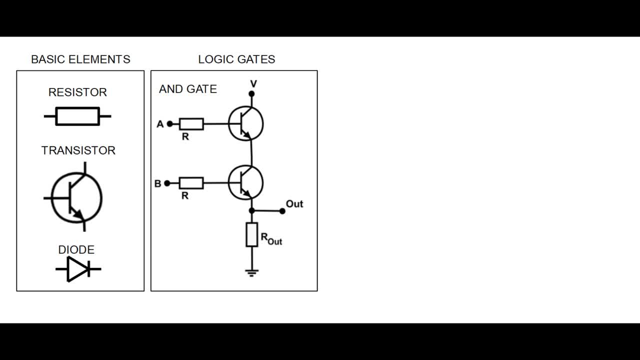 from analog electronics to digital electronics. Here, for example, you can see a logic AND gate that is made from two transistors and three resistors. Let's suppose that we have connected the plus 5 volts to the collector of transistor T1. If there will be zero volts on input A and 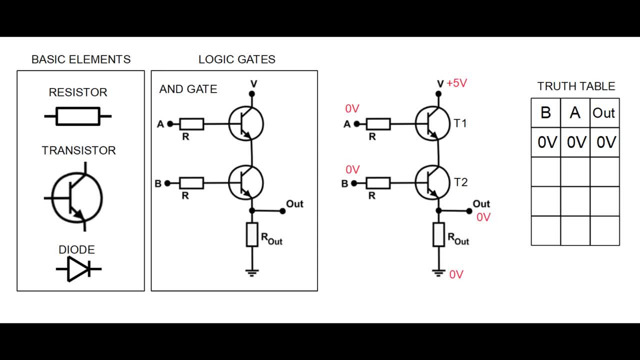 input B, there will be zero volts also in output. If we will change the voltage from zero volts to plus 5 volts on input A and leave the voltage on input B zero volts still in output, we will have zero volts. Also in case if there will be zero volts on input A and plus 5 volts on input B. 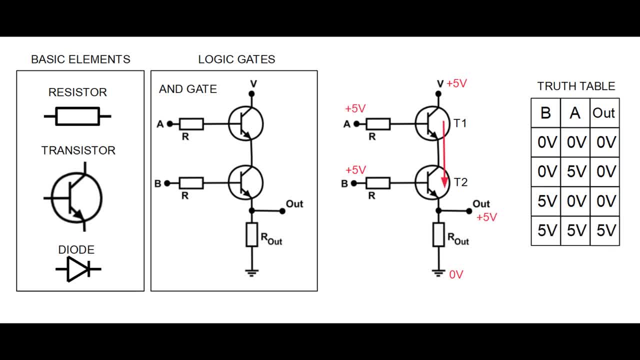 we will have zero volts in output. But now, if we change the voltage on both inputs to plus 5 volts, we have also plus 5 volts in output, because both of the transistors are in opened state. While changing these voltage levels, I also filled out this table with the corresponding voltages. 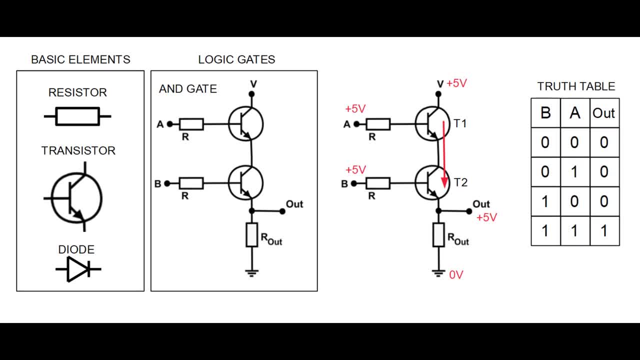 for both inputs and output, Now replacing zero volts with zeros and plus 5 volts with ones, we get this called truth table, and this is where digital electronics starts. In digital electronics, there are only high and low logic levels, and those are those zeros and ones that you can see in this table. 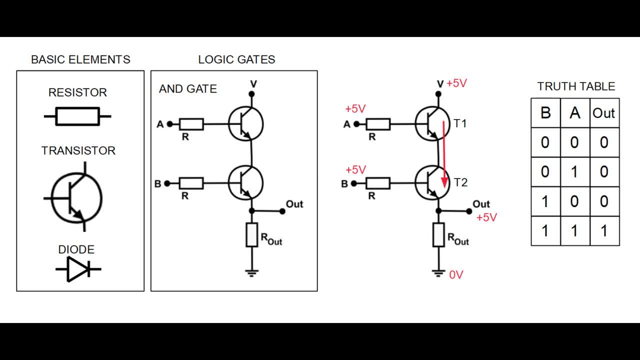 What's interesting is that we can describe this truth table using an equation, and in this case we can use an equation: input A multiplied by input B equals output. And indeed, if we multiply zero times zero, we get zero. if we multiply one times zero, we get zero if we multiply zero times. 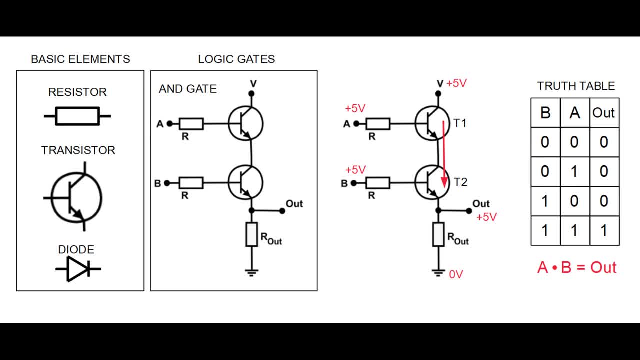 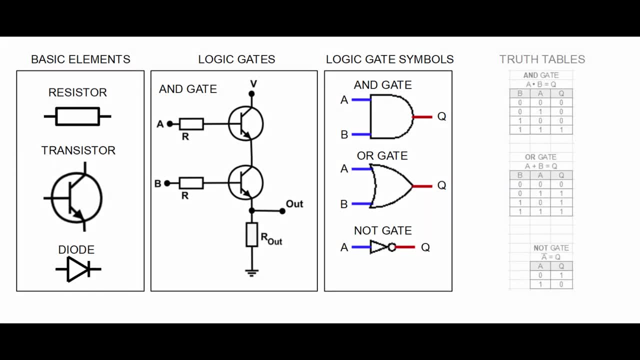 one, we get zero, and if we multiply one times one, we get one. In digital electronics, there are multiple logic gates, and each gate has its own truth table and its own equation. I have to say, though, that mathematics used in digital electronics is different from regular mathematics, and it is 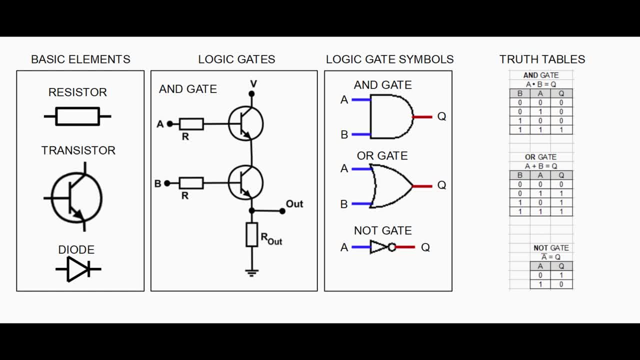 called boolean algebra. What boolean algebra allows us to do is to describe digital circuits using mathematical equations, and it is very useful in describing complex digital circuits and simplifying them. Now, using these logic gates, we can create more complex structures that are capable of adding. 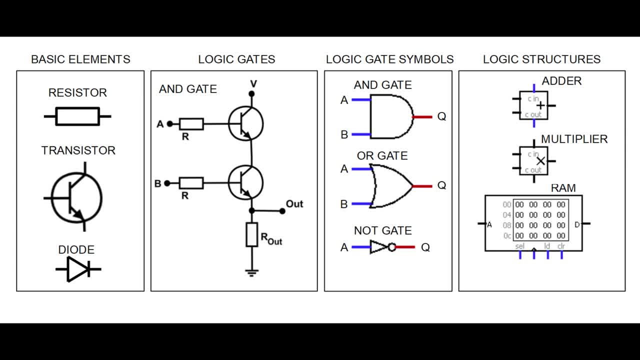 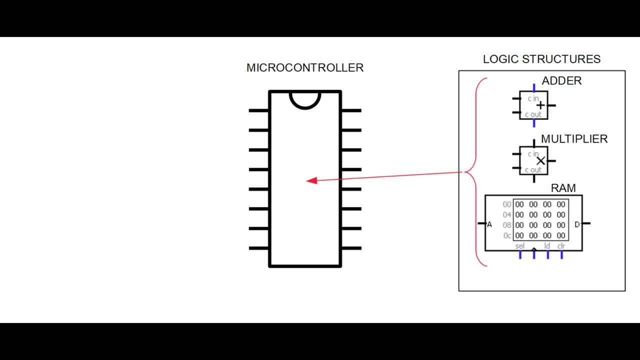 subtracting, multiplying and even storing digital information. These are the type of structures that are inside the microcontroller and it is possible to control them by using something called program. Program is stored inside microcontroller's internal memory and it can be transferred into microcontroller through programming pins that are specially made. 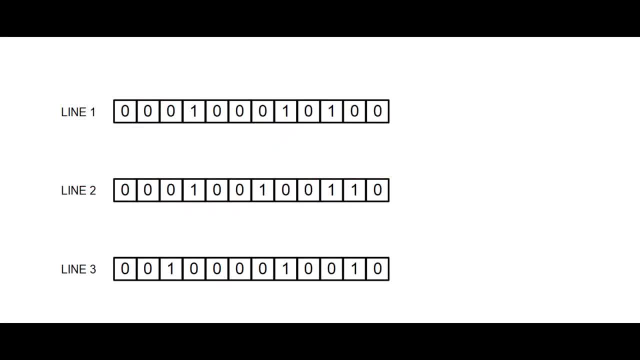 for this purpose. You can think about program same as you would think about lines of zeros and ones. Each line of the program has a predefined length and each part of the line has its own meaning. This won't be an actual program, but it should serve as a good example. 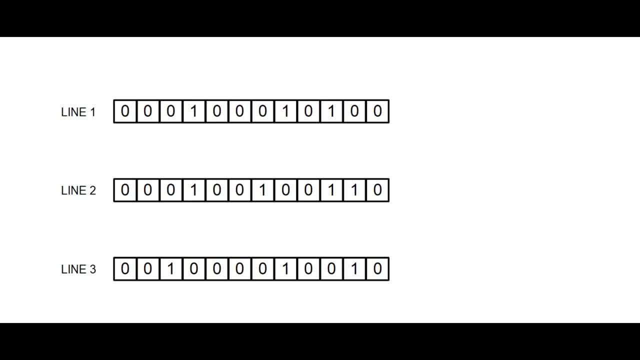 to better understand how the program is read by the microcontroller, Because lines of the code are always read in a certain sequence by the microcontroller. we will go through the program, starting from line 1, followed by line 2 and followed by line 3.. 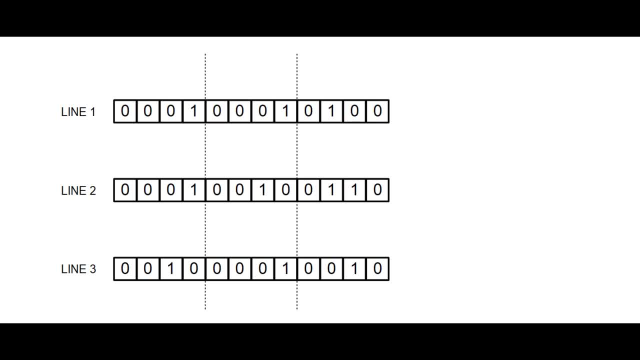 First, let's split all the lines in three parts. This first part is the line 2 and this is the line 3.. The first part of the first line will be a write operation, So it means that we will write some information in somewhere. 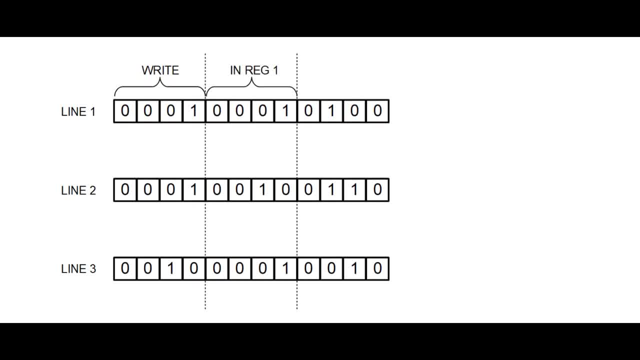 This second part of the line will tell us where we will write this information, and in this case, we will write it in a register 1.. If you are wondering, what is a register, register is simply a memory cell that is capable of storing some information. And now we come to the third part of this first line. 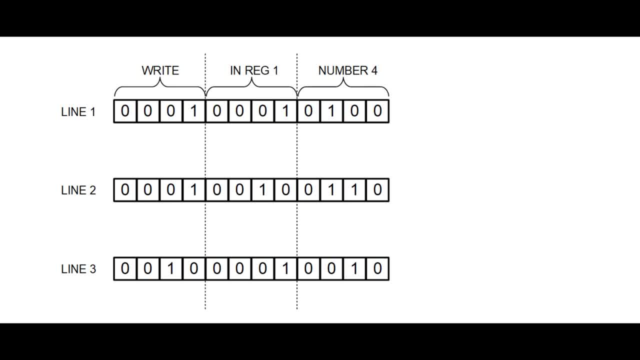 and it tells us what kind of information we want to write in register 1.. And in this case we want to write number 4.. If we would convert 0100 from binary to decimal numbers, then it would be number 4.. So if we go one more time over this first line of code and what it says to the microcontroller, 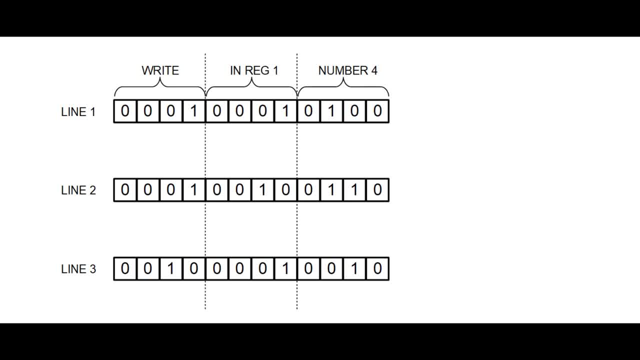 it says: write in register 1, number 4.. And so we come to the second line of code, And in this case, again, it will start with a write operation. The second part of the code will tell us in which register we want to write this information. 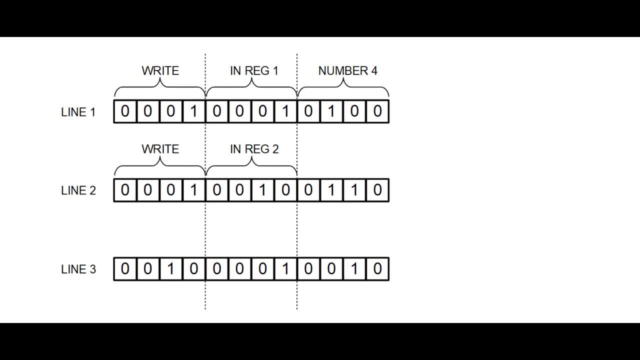 In this case, we want to write this information in register 2. And the third part of the code will again tell us what kind of information, what kind of number, we want to store in register 2.. And it will. in this case it will be number 6.. 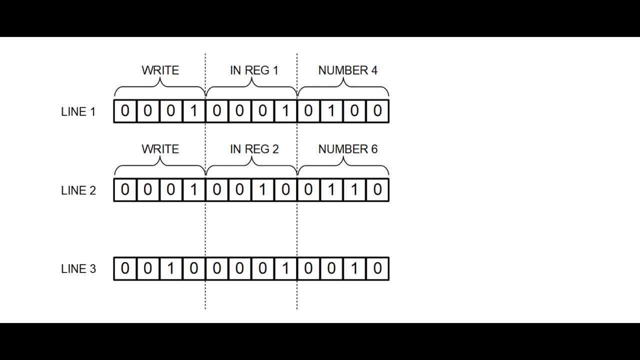 If we would convert 0110 from binary to decimal, it would be number 6.. The third line of code will start with a different operation. In this case it will be an add operation And what we will add. We will add the number that is in register 1 to the number that is in register 2.. 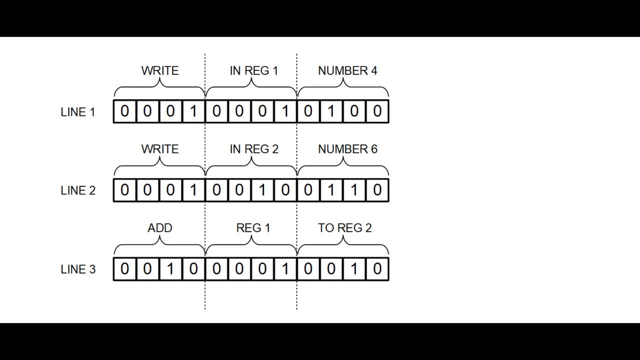 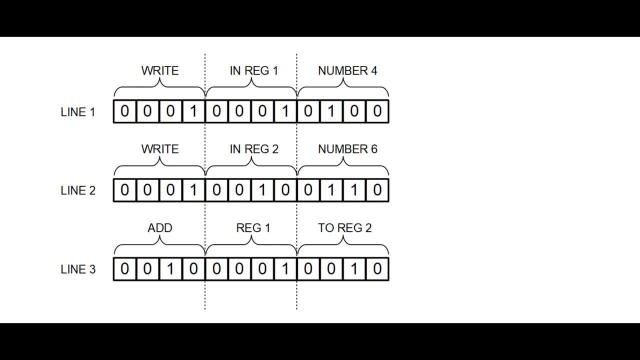 So what we get as a result after executing these three lines of code? we get the sum of number 4 and number 6 in second register, and that would be number 10.. If we would convert 1010 from binary to decimal numbers, then it would be number 10.. 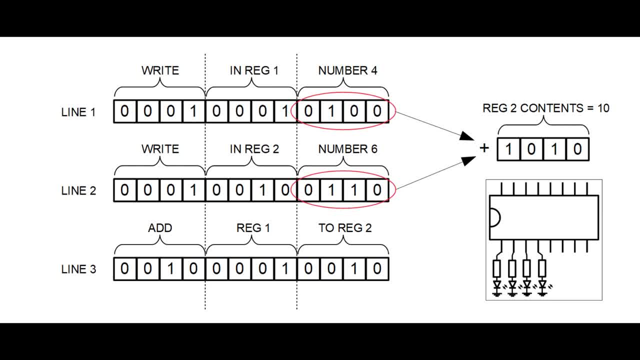 Now what we could do if we would want. for example, we could display the result using led lights that are connected to the microcontroller. Of course, as I said before, this is not an actual program, but this is approximate example how these lines of code are executed by a microcontroller. 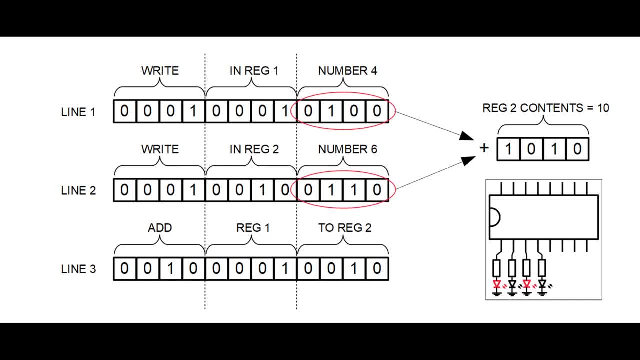 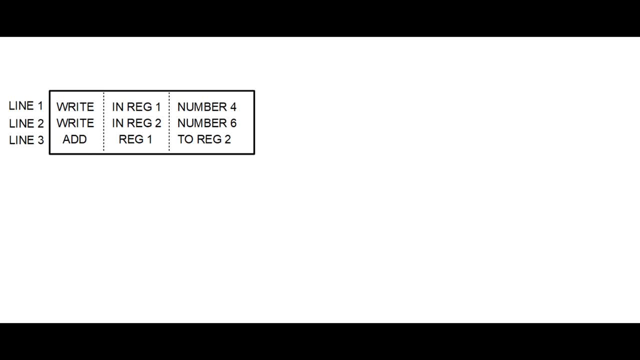 Now let's remove these binary codes and leave only those written words. What we get here is something similar to assembly language. What is an assembly language? it is a very low level programming language. As you can imagine, it would be very difficult for a human to memorize what each string of zeros and ones means. 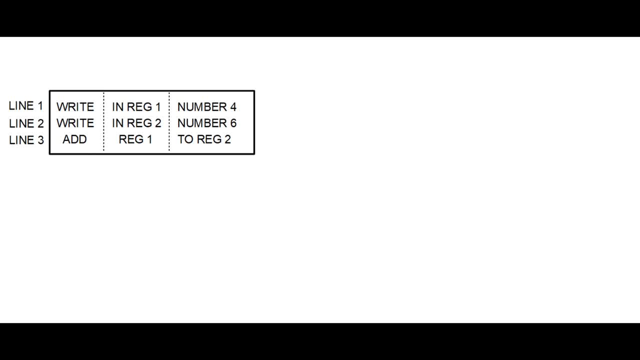 To make the job of programming easier, people have replaced these zeros and ones with written words and numbers that are a lot more meaningful for a human. Therefore, it becomes a lot simpler to write a program When the program in assembly language is finished and we want to burn it in. 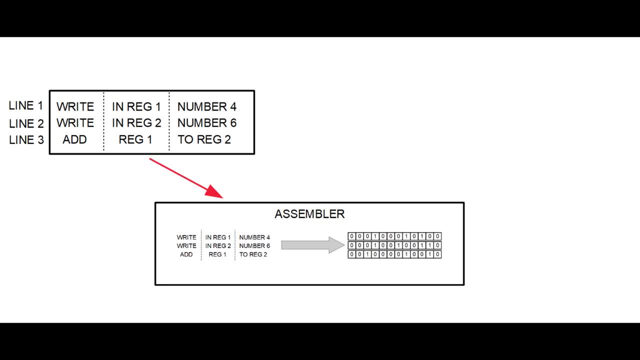 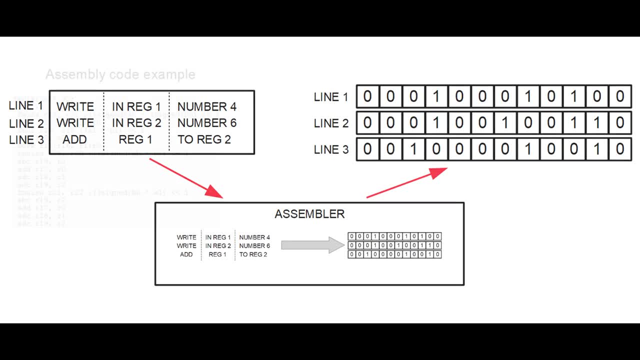 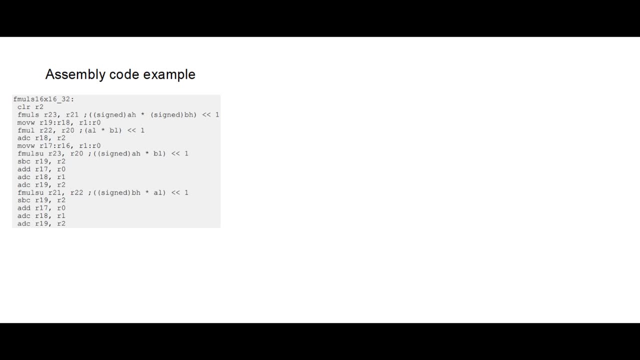 microcontroller. we are using something called assembler that converts our assembly code into zeros and ones that can be understood by the microcontroller. Here will be an example of an actual assembly code, Although it is a lot easier to write a program using this kind of language instead of zeros and 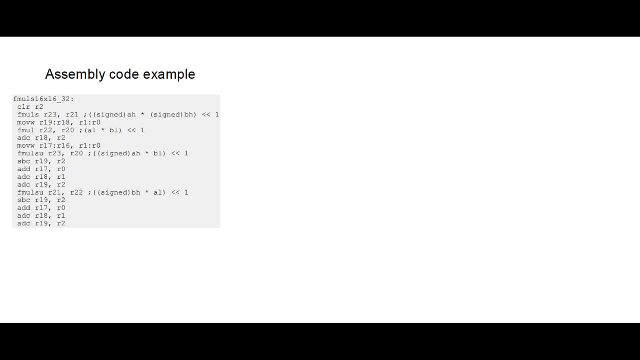 ones. it is still very difficult to write large and complex programs, and you also have to understand very well how the microcontroller is built and how it works. This is why there are a lot of other programming languages. that simplifies the job of programming even more. 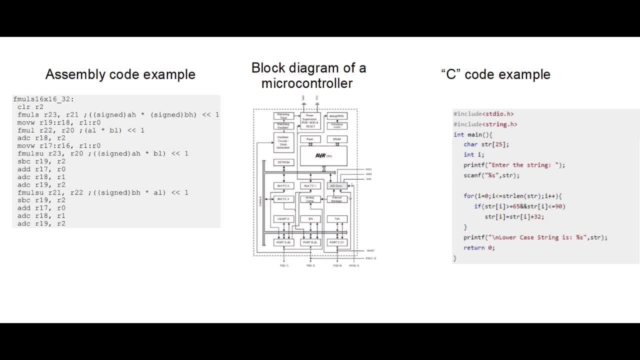 Some examples would be programming languages like C and C++. The main benefits of these languages are that they are easier to understand and they greatly reduce the time needed to create a program, Because, for example, what can be done in assembly language using 5 or 10 lines of code? it can be. 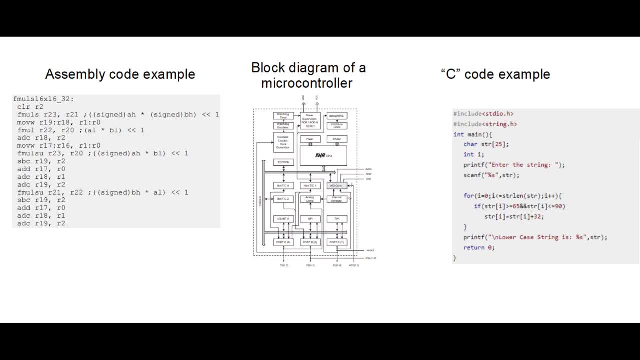 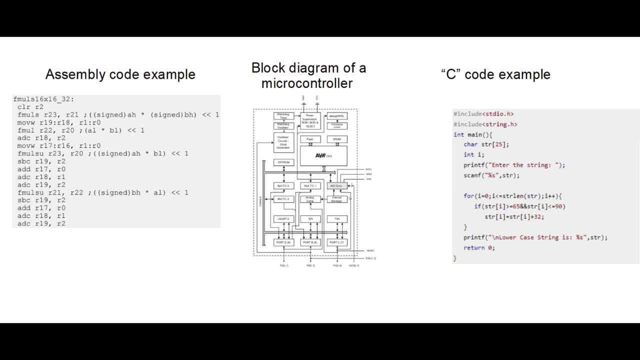 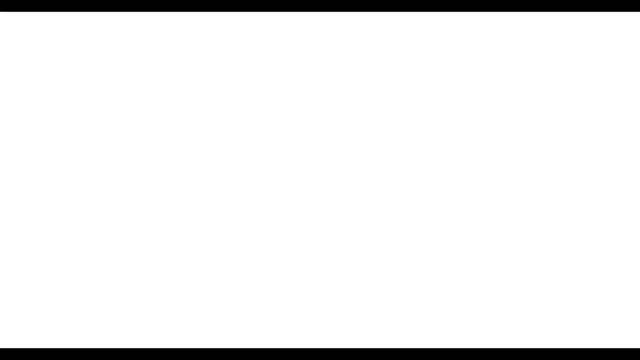 means that you don't have to understand the hardware as well to be able to create a program. The number of applications where microcontrollers can be used is endless, and it greatly depends on your imagination. For example, you can take a microcontroller, add some buttons and some lcd screens and create a 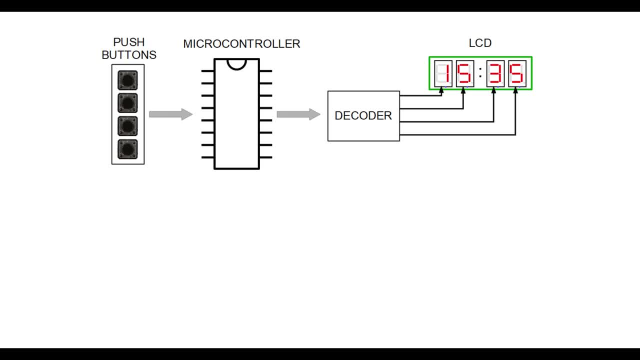 digital clock. Microcontrollers are used in everything, starting from children's toys and ending with that refrigerator that stands in your kitchen. Now you should have a better understanding what is a microcontroller, how it works and where it can be used. If you like this video and if you want to help me grow my channel. 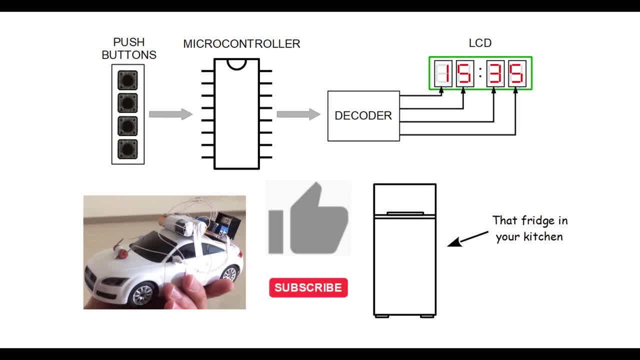 consider smashing that like button and subscribe for more of my content. Cheers, guys, and stay smart. wwwmicrosoftcom.